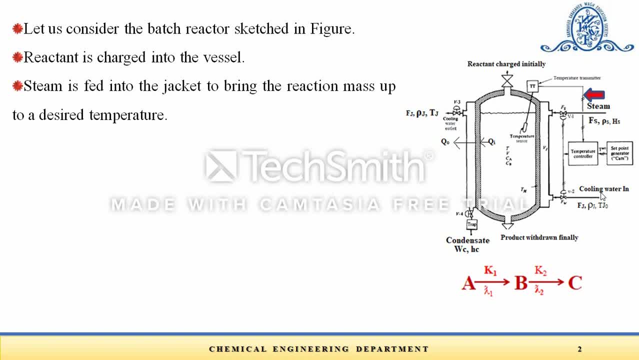 Fs having density, rho s and enthalpy hs. The steam is provide a heat to the reaction mass to bring that reaction mass up to desired temperature and then that steam get condensed and it is separated from the bottom of the jacket with feed rate. Wc having enthalpy hc. 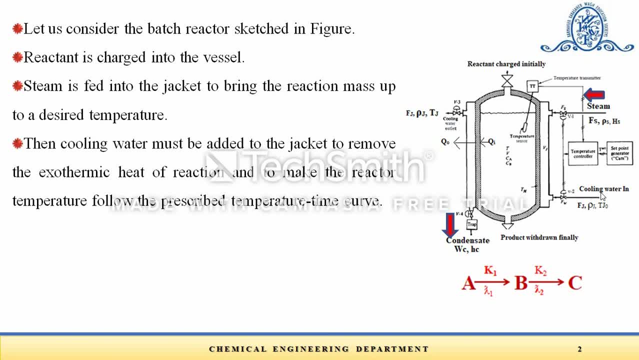 Then cooling water must be added to the jacket to remove this exothermic heat of reaction and to make the reactor temperature follow the prescribed temperature time curve. So here cooling water inlet with a flow rate Fj density is separated from the bottom of the jacket with feed rate Wc having enthalpy hc. 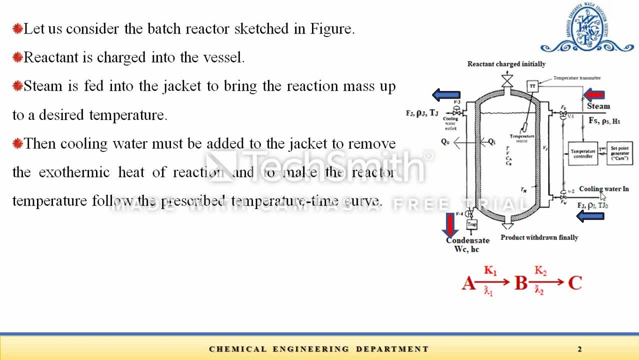 Same flow rate of cooling water is out, that is Fj, and density rho j, but the temperature is different, that is Tj. This temperature profile is fed into a temperature controller as a set point signal and that set point varies with a time. The first order constitutive reaction takes place in the reactor as a time. 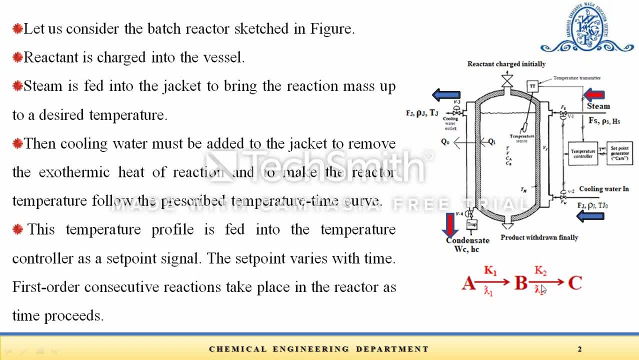 And here that constitutive reaction is: A gives B and B gives C. with reaction rate constant, k1 and k2 particularly, and with exothermic heat of reaction lambda1 and lambda2 respectively, The product that we want to form is component B. If we let the reaction go too long, then 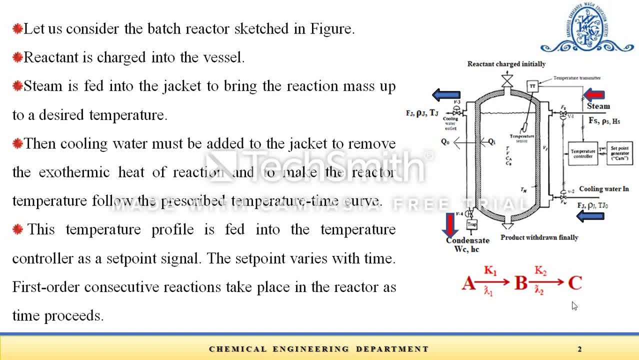 too much of B will react to form undesired product C. that is, conversion of A will be maximum, but yield of desired product B will be low. On the other hand, if we stop the reaction too early, too little of A will react. that is conversion and yield- both will be low in this case. 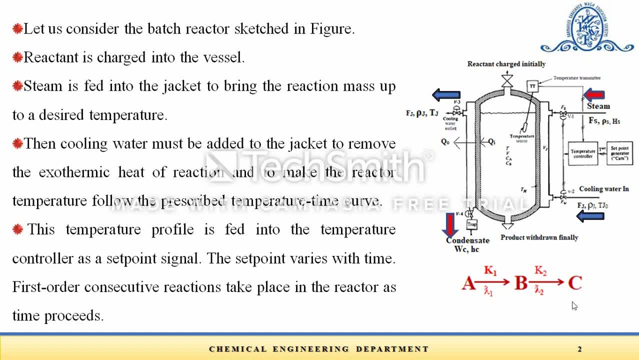 So there is an optimum batch time when we should stop the reaction and this is done by quenching, that is, sudden cooling. So we have to focus on kinetics, that is, values of rate constant, k1 and k2.. So here we will be interested in keeping k1, reaction rate constant, or we can say that: 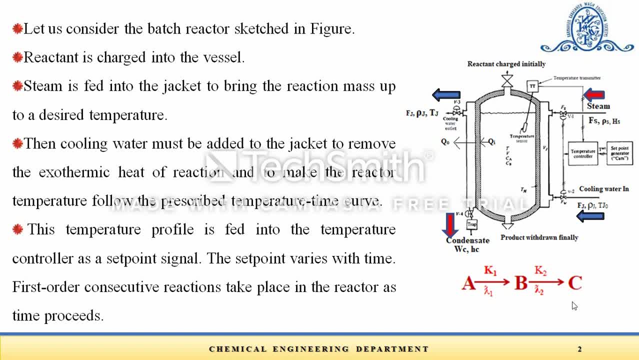 its value will be more than that, more than production of for the desired product B as compared to the undesired product C. So with this background, let us derive the mathematical modeling for the batch reactor. So we will make some assumptions: Constant density system, perfectly mixed reactor content, constant heat capacities. we neglect. 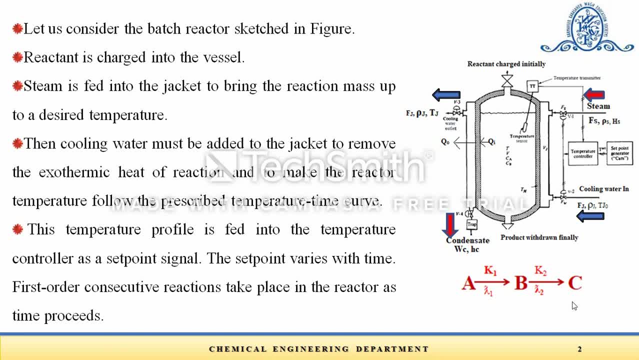 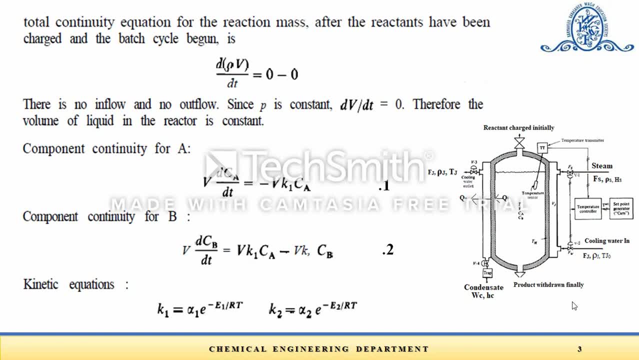 the heat losses and also the jacket metal wall capacitance will also negligible. So here, first of all, we will concentrate on the reaction mass. Total continuity equation for the reaction mass after the reactant has been charged and the batch cycle began is: d by dt of rho into v is equal to 0 minus 0. that means there is 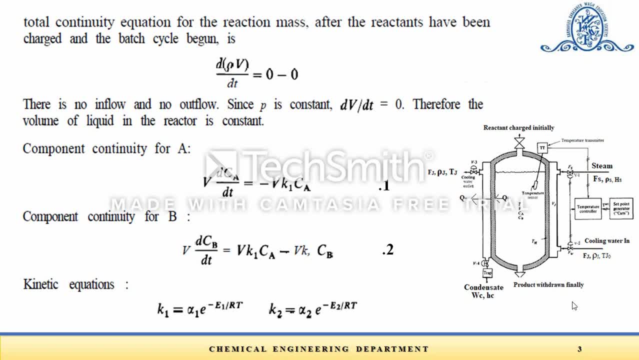 no input, no output. So the accumulation term will be 0. that is, volume of the system remains the constant. Then we will see. Let us see. Then we will apply component continuity equation for the component A. We know the definition: accumulation of the moles is nothing but flow of moles of A into 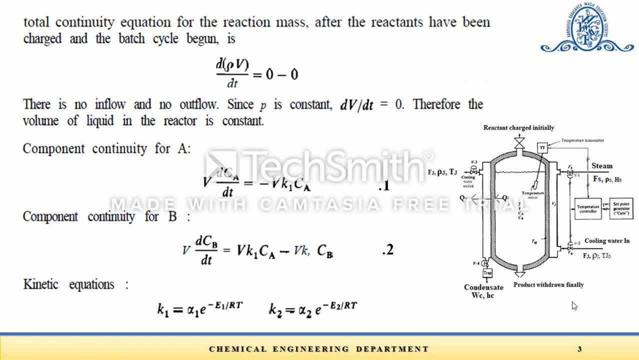 the system, minus flow of moles of A out of the system, plus rate of formation of moles of A inside the system. So inlet and outlet term will be 0 as a batch reactor. So here the first, that is the desired reaction is: A gives B. 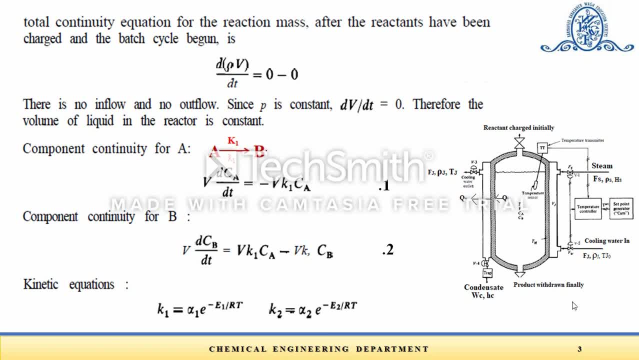 With reaction rate constant k1 and lambda 1 as a heat of reaction. So here rate of reaction for A is given by Ra is equal to k1 Ca, and that's why the rate of formation of A is given by minus v k1 Ca. 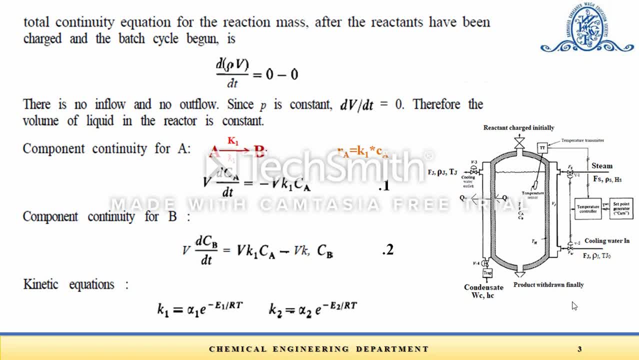 Minus sign is due to the component A is going to disappear and that is equals d by dt of v into Ca, v is taken, This, v is taken outside. So here we will have d. Ca by dt is equal to minus v. k1 Ca as a first modeling equation. 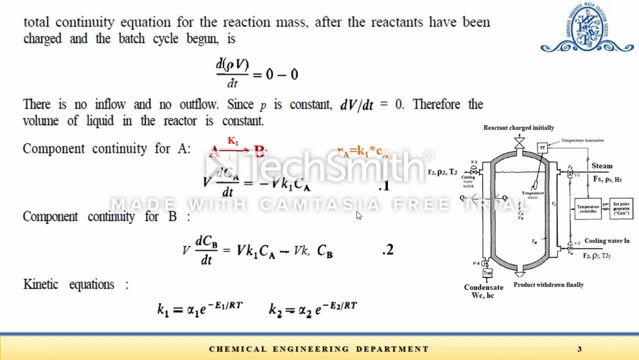 Similarly we can write a component continuity equation for component B and that component B is involved in two reactions: A gives B and B gives C. In first reaction it is a product, in second reaction it is a reactant. So here we can have rate of reaction for B. 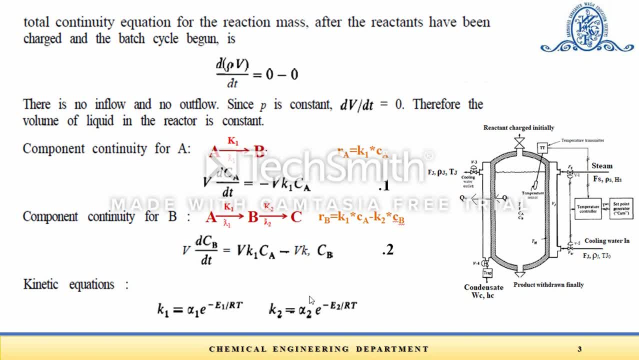 That is k1 Ca minus v k1 Ca. So here we can write component continuity equation for component B and that component B is involved in two reactions. Here we see a reaction of B minus k2 Cb. k1 Ca is due to rate of formation of B and k2 Cb due to rate of reaction of B. and here 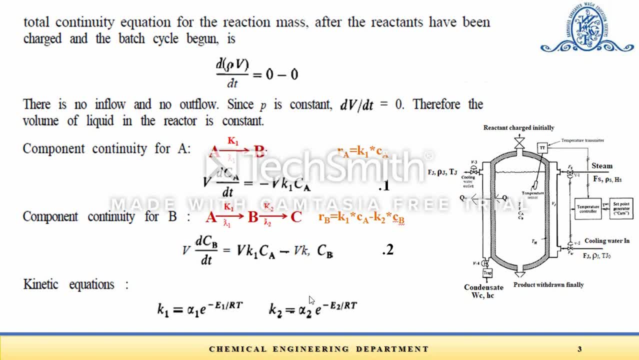 then the rate of formation of B can be given for this component continuity equation. that is v k1 Ca minus v k2 Cb, That is equals to that is d by dt of v into Cb. v is taken outside as v is constant. 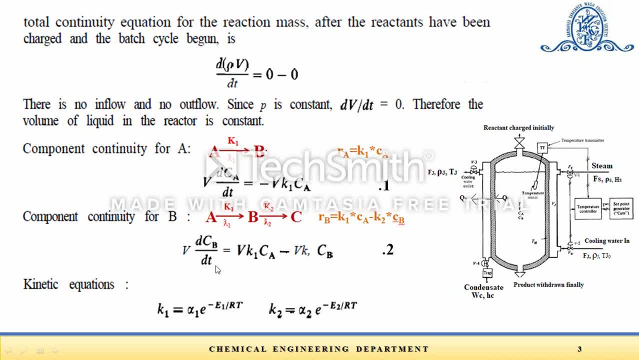 So this forms second modeling equation for this batch reactor. Minus sign is given by lambda 1.. Now equation 1 gives how CA is changing with respect to the time, and equation 2 gives us how CB is changing with respect to the time. 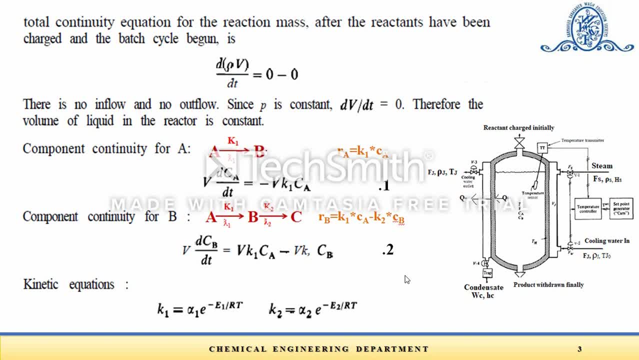 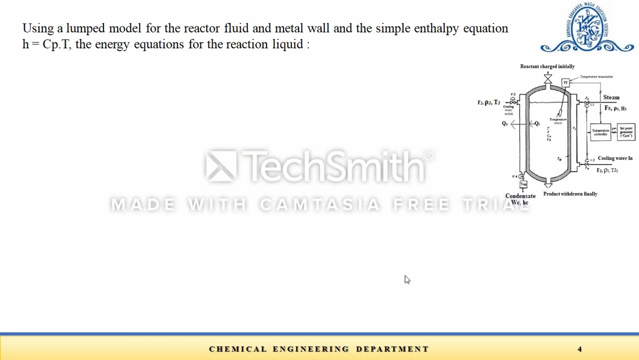 Now here, formation of CA and CB. that also depends upon the kinetics, as we have already discussed K1 and K2. So we should have K1 more as compared to the K2, and both are the function of temperature. Now we will apply lump model for the reactor: fluid and metal wall, that energy equation. 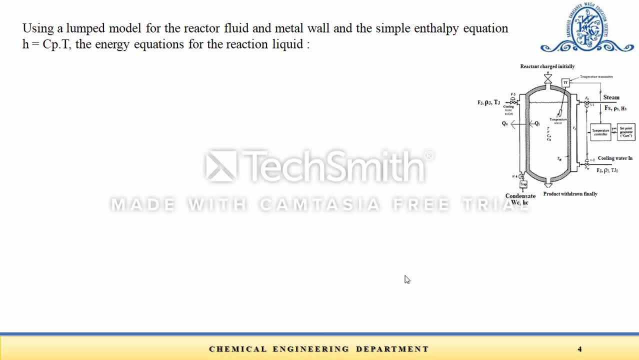 So simple we have. H is equal to. So energy equation for the reactor fluid can be defined as: accumulation is equal to heat evolved due to first reaction minus heat evolved due to second reaction plus heat transfer to the metal wall. Now flow of energy in and flow of energy out. 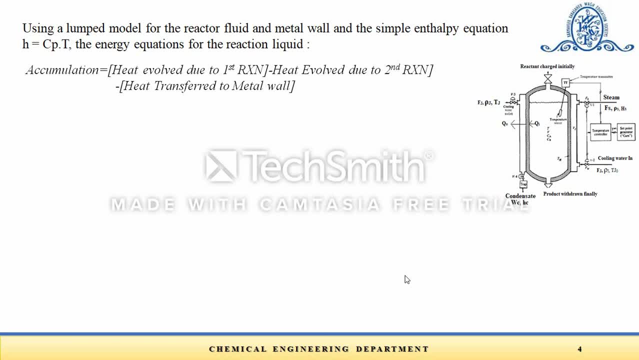 Due to bulk flow will be absent here because there is no inflow and outflow. Only heat added or heat evolved to the system is due to the exothermic heat of reaction due to first reaction and second reaction. By writing the different terms to the above equation, we will have Rho Vcp into dT by dT. 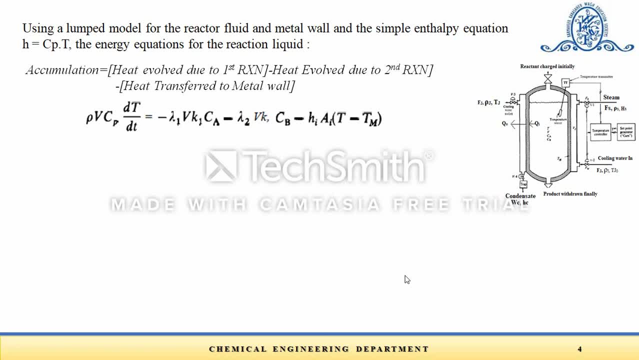 Rho Vcp is a constant, So it is taken out Outside Plus, or that is equals to minus. lambda 1, V, K1, C, A is the heat evolved due to the first reaction. That is, lambda times the rate of reaction first. 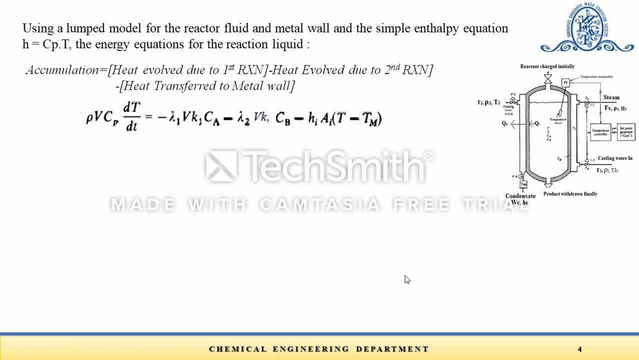 Minus lambda V, K2 C. V is the heat evolved due to the second reaction, that is, lambda 2 times the rate of reaction for V, and that is and minus heat transfer to the metal wall. So this heat transfer to the metal wall is nothing right. 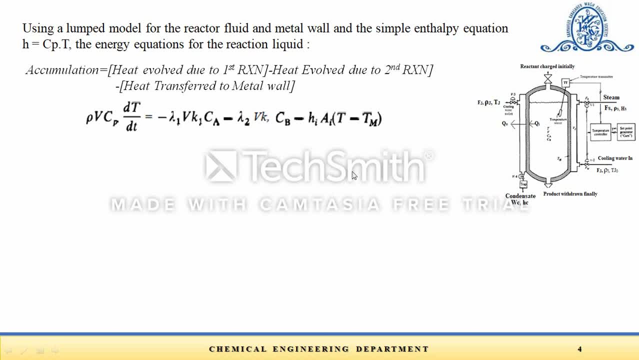 But the heat heat is transferred from the steam or the cooling water at the inside of the surface, this metal wall right Heat is transferred. that is QI. that is nothing but at inner surface. So HIAI heat transfer coefficient at inner side surface area at inner side. 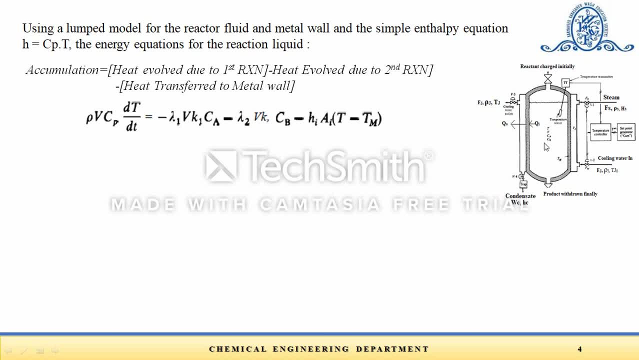 Now this T minus Tm is the temperature difference. So heat is given from inner side, that is exothermic heat of reaction. That is why T minus Tm. it is given from reaction mass to the metal wall. That is why T minus Tm. 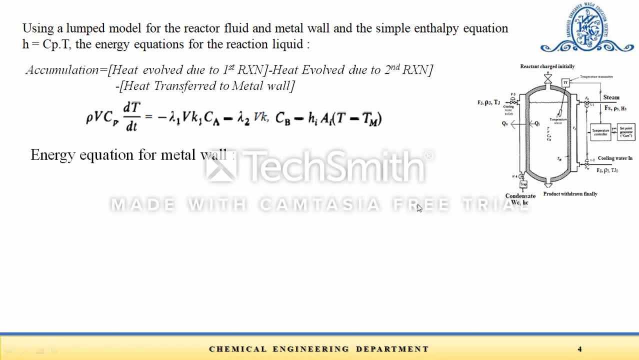 Similarly we can write the energy equation for the metal wall. For the metal wall there is no inflow, no outflow of the fluid. Similarly, there is no exothermic heat of reaction carried out in the metal wall. So this term also neglected this two term. 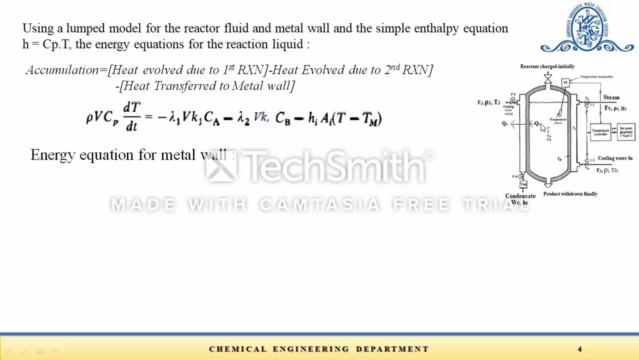 Only heat transfer at Inner surface, that is QI, and heat transfer at outer surface, that is QO. These two term will be there So we can write the define the equation that is: accumulation for the metal wall is equals to heat transfer at outer surface minus heat transfer at inner surface. 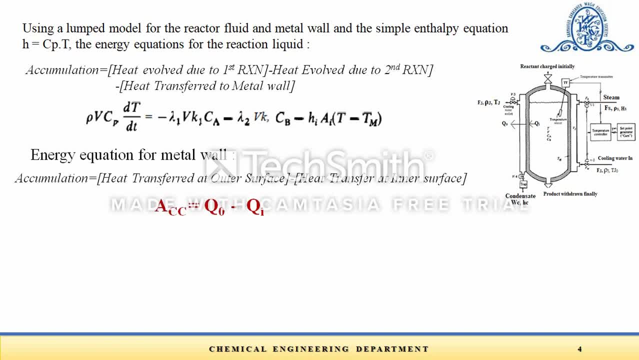 So here accumulation is nothing but QO minus QI, and we know Q is equal to HA delta T, right? So here we can write the terms for this energy equation. for metal wall Accumulation, This term is nothing but Rho, M, Vm, Cm. 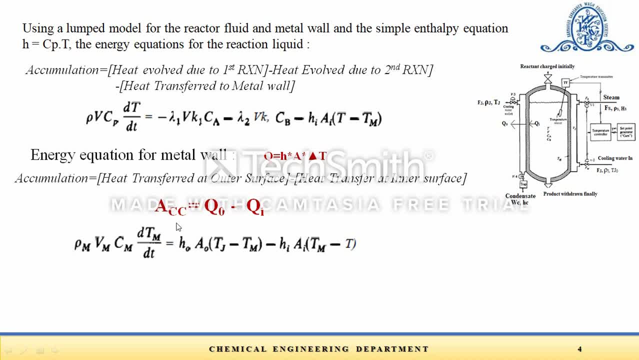 So all these terms are constant. So we have taken it outside and d by dt of Tm, that is temperature for metal wall. Now heat transfer at outer surface is nothing but HOAO, Tj minus Tm. So at outer surface the temperature difference will be Tj, that is jacket fluid minus metal wall. 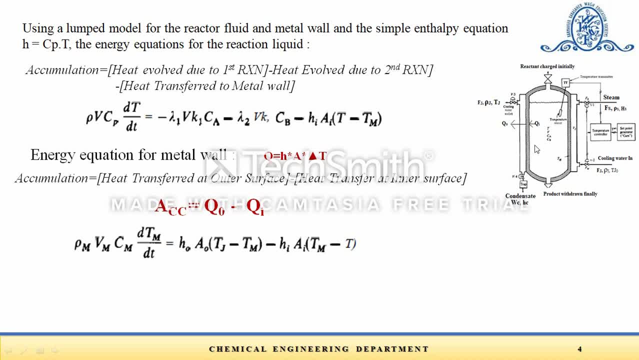 And at outer surface that is HIAI Tm minus T. So this is the temperature difference. So these equations for the metal wall, Where lambda 1, lambda 2 are the exothermic heat of reactions, for these two reactions, 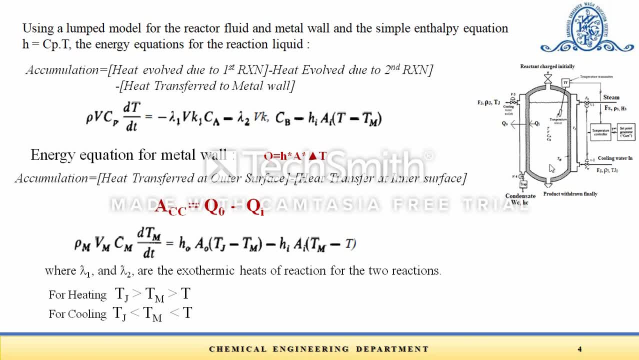 Now we have to notice that For heating, Tj will be greater than Tm, which is greater than T, And exact opposite sign will be there for all these temperatures. for cooling Now we have to keep in mind that outside heat transfer coefficient H 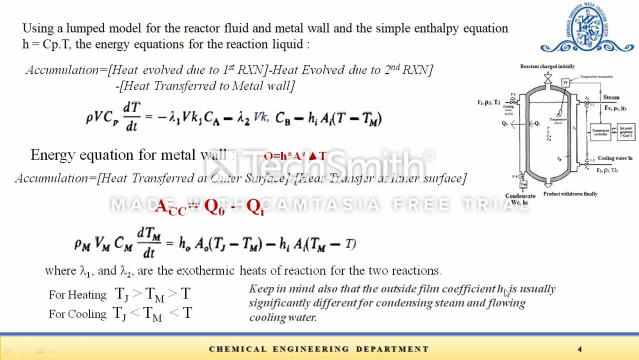 is also significantly different for condensing steam and flowing cooling water. That is important. So here, the equation 3 gives us how temperature of the fluid is changing with respect to the time, and equation 4 gives us how the metal wall temperature changes with respect to the time. 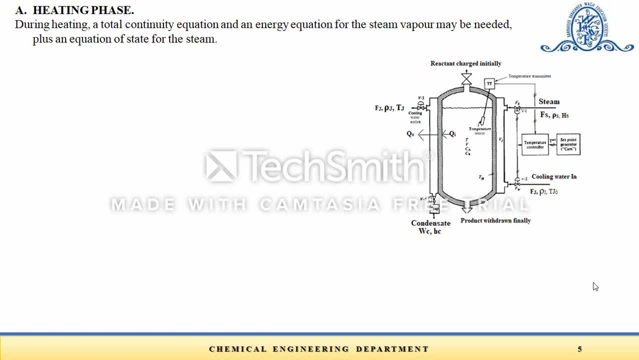 Now, to describe what is going on in the jacket, we may need two different set of equations, depending upon the stage, whether it is cooling or heating. We may even need to consider third stage, that is, filling the jacket with cooling water. But if cooling water flow rate is high, 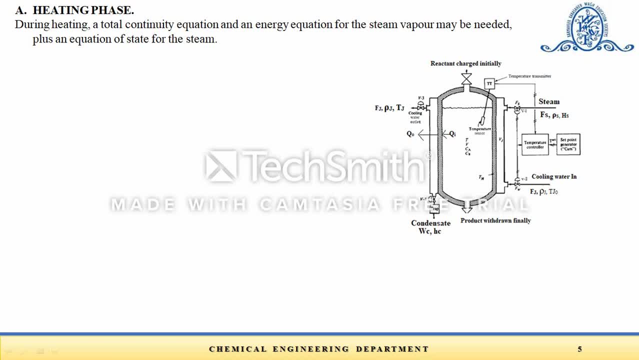 and the jacket volume is low or small, the time to fill the jacket may be neglected. So here we have two different set of equations. One is cooling water and the other is heating. So here we have two different set of equations: One is cooling water and the other is heating. 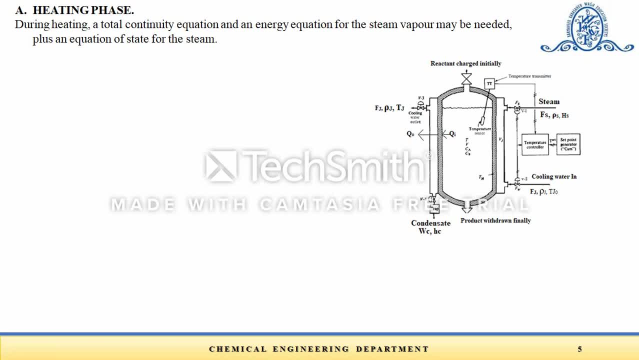 So here we will see, or we will form the model for heating phase and cooling phase. Now concentrate on heating phase. So during the heating, total continuity equation and energy equation for the steam and one more equation of state for the steam we have to model 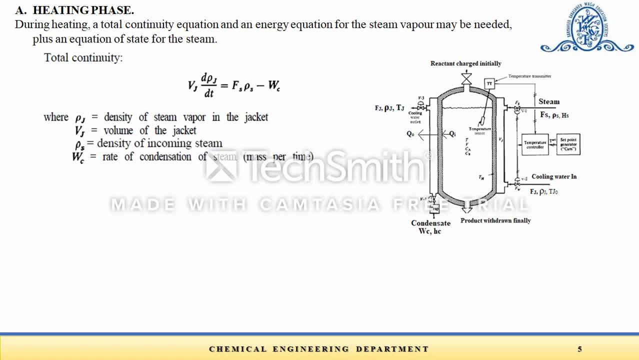 Now total continuity equation. So here for total continuity equation. the flow of steam in or minus flow of steam out is equal to accumulation of mass of the steam. So here we can see this flow of steam in is nothing but, or flow of mass of steam in is given. 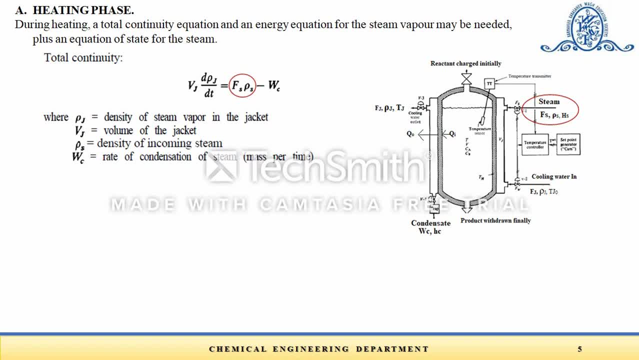 by Fs into rho s, where Fs is the volumetric flow rate minus flow of condensate out of the steam. So here we can see this flow of steam in is nothing but, or flow of mass of steam in is given by Wc.